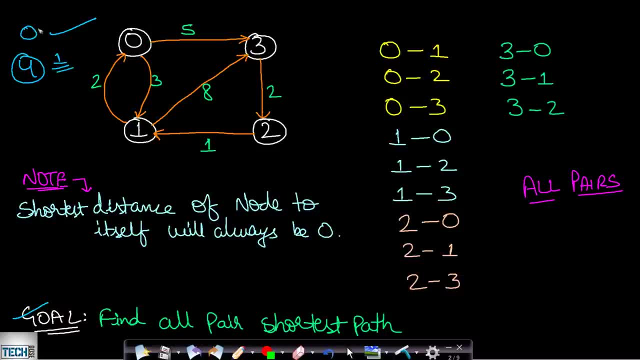 vertices. okay, so one will be itself, that is, from zero to zero, for this node zero, and the others will be from zero to one, zero to two and zero to three. so like this for a graph having v number of vertices. for each and every vertex they it will be having v number of options. so this is including. 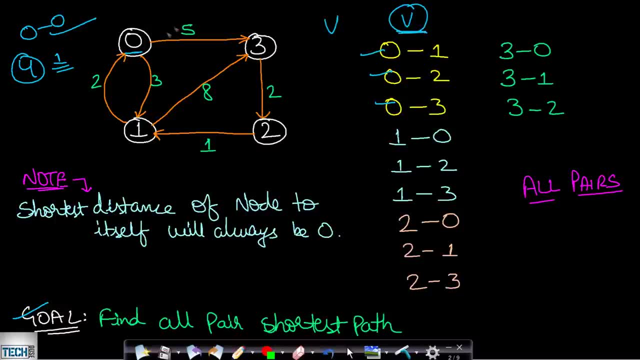 itself. in this case, if we exclude the self loops, then we will be having three number of pairs for each and every vertex. that is, if we have v vertices in a graph, then we will be having v minus one number of pairs if you exclude the self loops. okay, so these are all the pairs for. 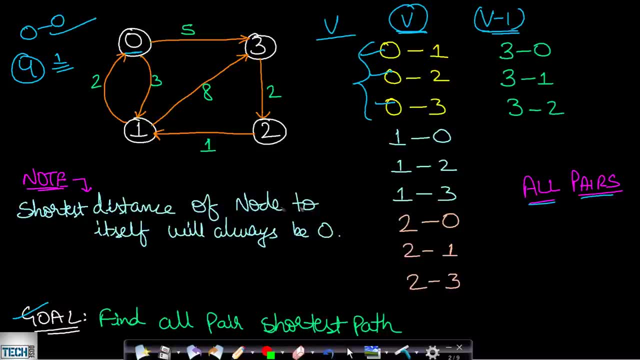 the given graph. now, one thing to note is: the shortest distance of a node to itself will always be zero. so if we want to find the shortest distance from zero to zero or from one to one, then they will always be zeros, since our starting position and the ending position are both same. 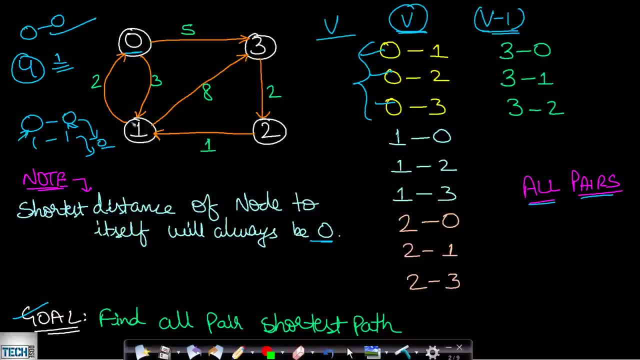 therefore, cost will always be 0 in this case. now, if you want to find, let's say, the shortest distance from 2 to 0, then it will come out to be this: 1 plus 2, which will be 3. okay, so i hope you understood what we actually need to find. if 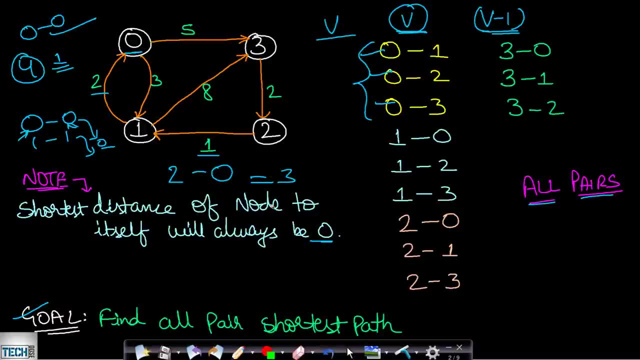 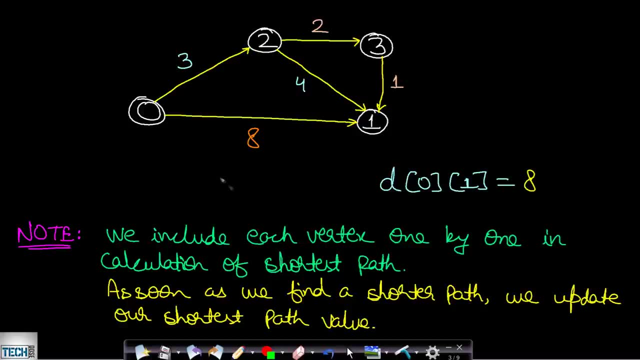 we are given this graph. we want to find the shortest path between each and every pair of vertices in the given graph, so this is known as all pair shortest path. now, having seen the problem statement, let us assume that this is our given graph. in this case, if we know the distance from: 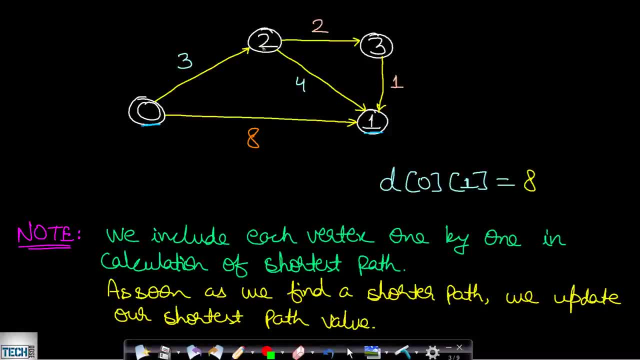 0 to 1, we do not know anything. we have knowledge just about the adjacent distances. okay, so in this given graph we know only about the adjacent distances. so from 0 to 1, we know that the distance is 8, so the distance of 0 to 1 is 8.. now let us include this node 2 and see if we 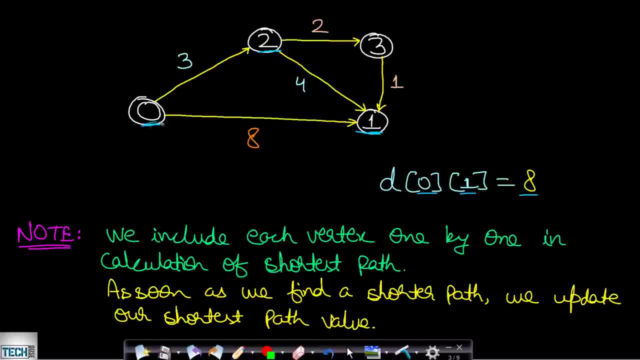 have an alternate, lower cost path in order to reach to this one from this 0. so we have a path via this two, which is of cost 3 plus 4, which will be 7.. so, already known cost from 0 to 1 is 8. 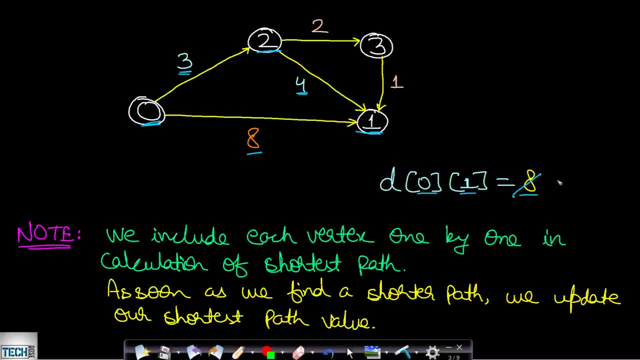 and the new cost is seven. so since seven is lower, we can replace this cost and write here seven. okay, now let us include the other vertices as well. so the other vertex is three. if we include this three, then let us find out if there is any path which will lower our cost. so if we include 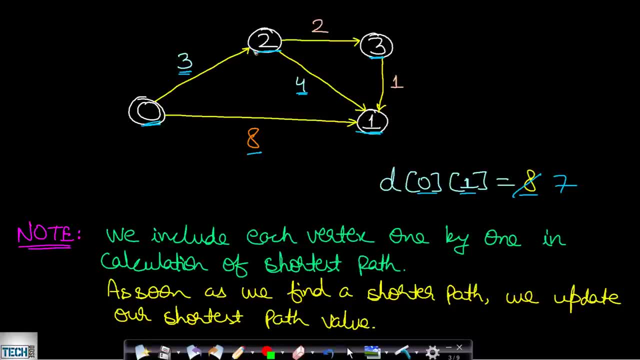 this three. then there is another path, which is from zero to two, from two to three and from three to one. so the total cost is three plus two plus one, which will be six. now, since six is lower than the already known cost, which is seven, therefore, we will be replacing it with six. now there are 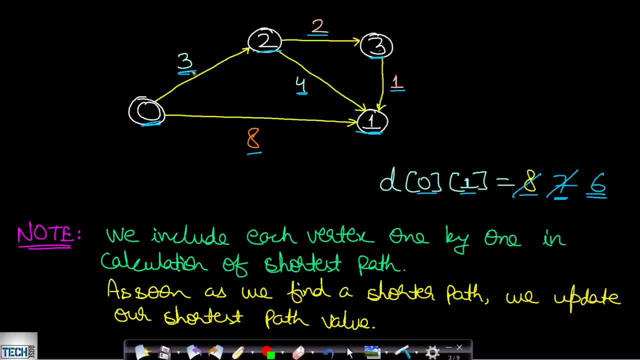 no other vertices to get included, and so, after including all the vertices one by one, we will be having the shortest cost, from zero to one in this case. okay, so like this, we will be updating for all the pairs of vertices, and so at the end of the operation, after including each and every, 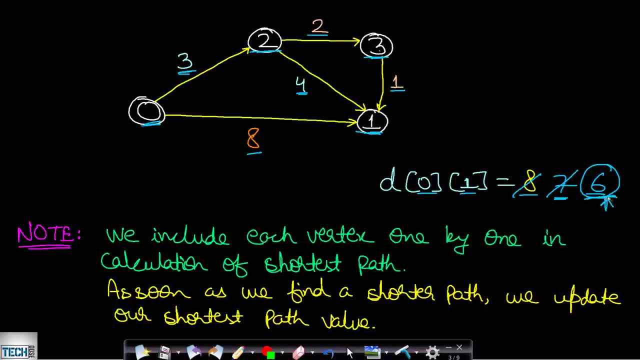 vertex, we will be getting the shortest path at the end. so this is the entire logic of this algorithm i have just shown for a single edge in this case. okay, that is just for a single pair. now, the thing to note here is we include each vertex one by one in the calculation of the 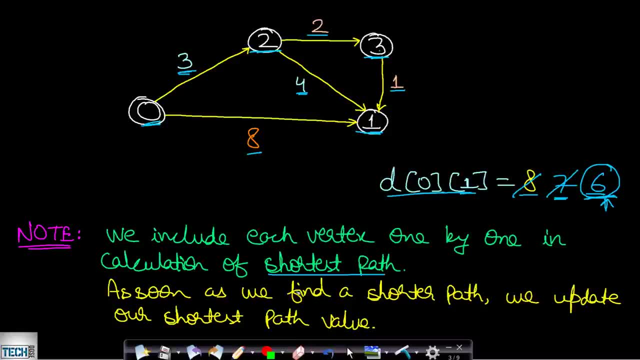 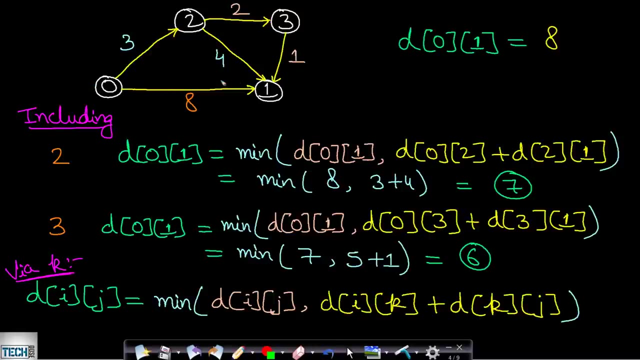 shortest path, like i have shown here. okay, as soon as we find a shorter path, we update the shortest path value. okay, so this is one such example. this is just for a single pair, from zero to one. now i have taking the same example and let us solve it mathematically. so in this case, we had already 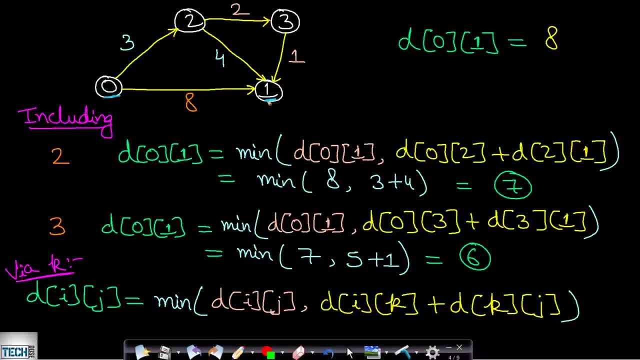 assumed that we want to find the distance from 0 to 1 and initially we only know the adjacent vertices distance. so we just know that from 0 to 1 the distance is 8.. now i have already written here 8. now we will try to include all the other vertices and we will try to optimize the shortest. 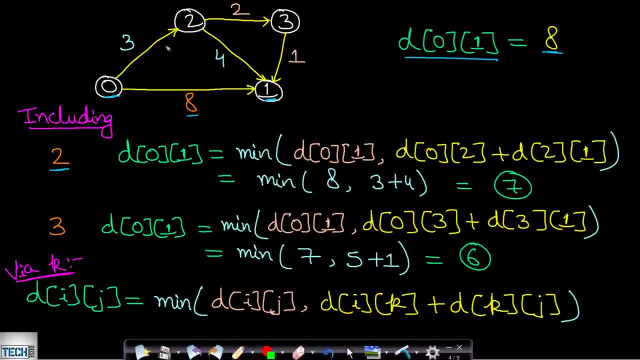 cost path. okay, so in this case, if we include this node 2, then, as i had already said, the distance of 0 to 1 will be equals to minimum of the already remembered distance, which is 8 comma, the new path distance, which will be from 0 to 2 and 2 to 1, so this will be 3 plus 4.. so this is 3 plus 4, and now 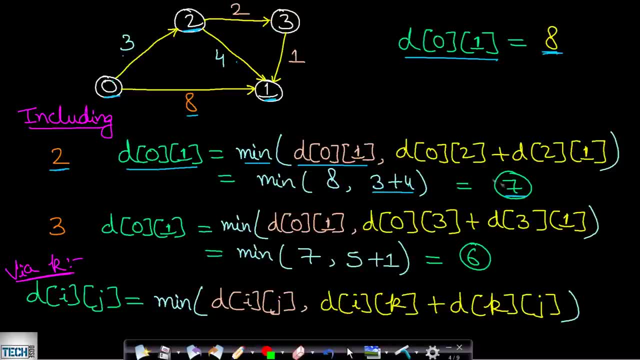 you can see that 3 plus 4 is lower, so it will get updated to 7. okay, now we will try to improve the distance from 0 to 1 and include the other vertices as well. so the other vertex is 3.. so on. 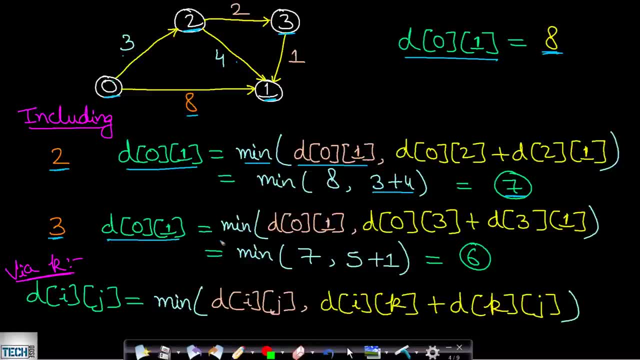 including 3. we want to actually find the shortest cost from 0 to 1. that will be equals to the minimum cost which is already stored, so in this case it will be 7 now and the cost from 0 to 3 plus 3 to 1. so from 0 to 3 the cost will be 3 plus 2, which will be 5, and from 3 to 1 the cost is 1. 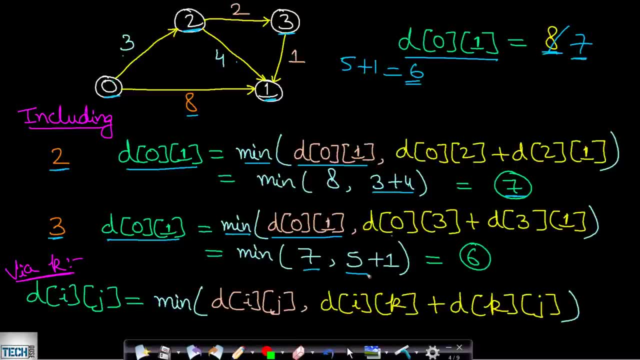 so the total cost will be 6 and the already stored cost is 7 and the cost will be 6.. so the cost will be 6 and the cost will be 6.. so this cost will again be replaced with 6.. so this is the algorithm for finding the shortest path between two vertices. 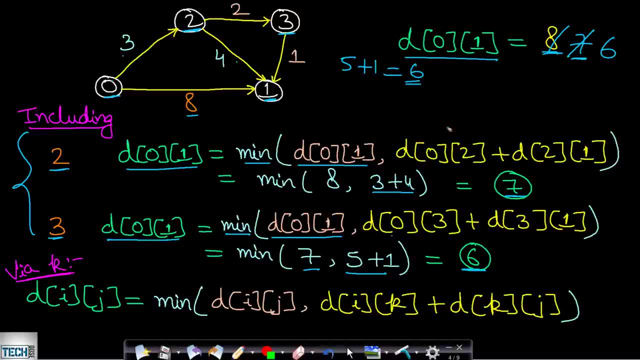 so in this case we will be calculating the shortest path among all the pair of vertices. now this entire formulation can be generalized. let us say, if we are including the kth vertex, then the distance from i to j will be equals to minimum of the already known distance from i to j. 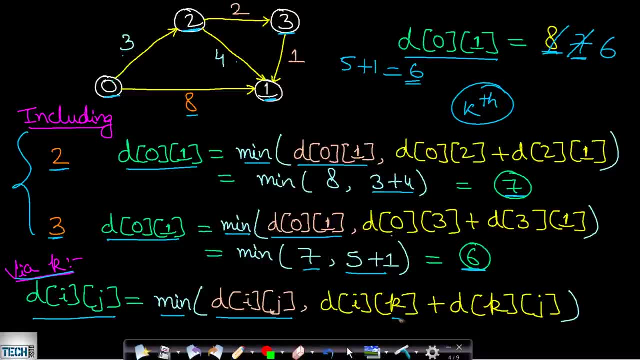 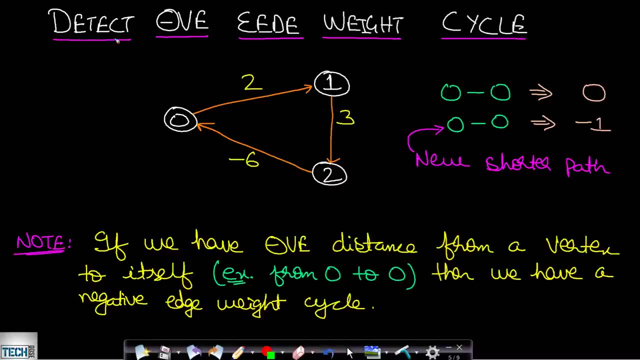 alternate path which we will be having after including the kth vertex, which is from i to k plus k to j. so i hope this is a very simple formulation in order to understand. so this we will be using in this entire algorithms. now, one important thing to note is floyd-warshall can. 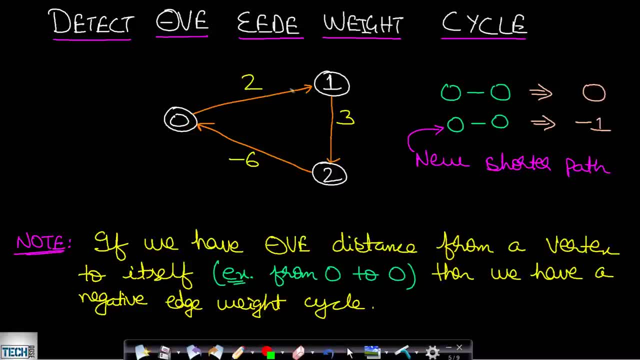 detect negative edge weight cycle. so let us assume that this is our graph. and now, in this case, if you start from zero and you want to find the cost from zero to zero, then it will be zero. now, if you try to calculate the alternate path cost, which will be from zero to one, from one to two and from. 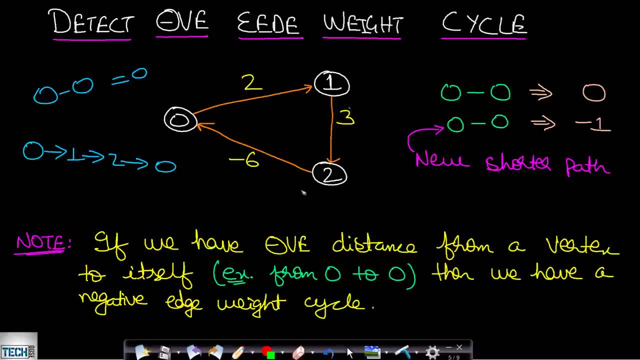 two to zero. this will be two plus three, three plus minus six, and this will come out to be minus one. so you can see that this alternate path is having cost equals to minus one, and since minus one is lower than zero, this zero to zero cost will now be minus one. and as long as you keep repeating, 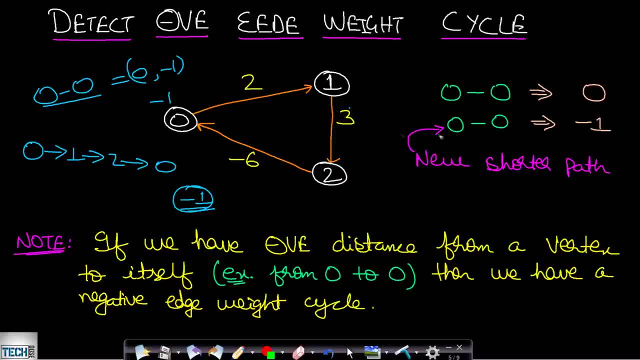 the cycle. it will keep repeating the cycle and you can see that this is the Zero to Zero decrementing. okay, so you can see that from the same vertex to the same vertex, the distance should always be 0, but since you have a negative edge weight cycle, therefore you are having weight. 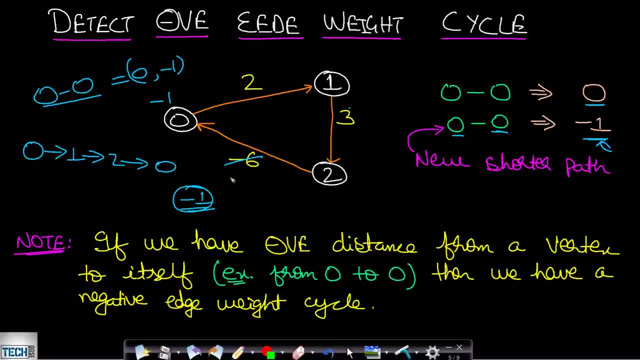 equals to minus 1. okay, now, if it was minus 4 instead of minus 6, then this will not be a negative edge weight cycle, because the effective edge weight should be negative. but in this case it will be 2 plus 3 minus 4, which will be 1, so this is not having effective edge weight negative. 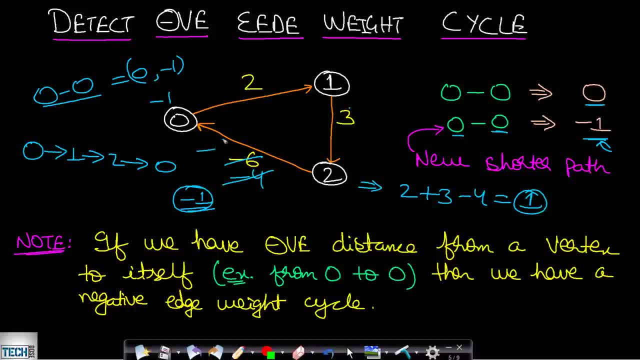 so this is not a negative edge weight cycle. but if it is minus 6, then this will be a negative edge weight cycle because the sum of the edge weights for this cycle will be negative, which is minus 1.. so this is a problem. so this floyd-warshall algorithm can detect the negative. 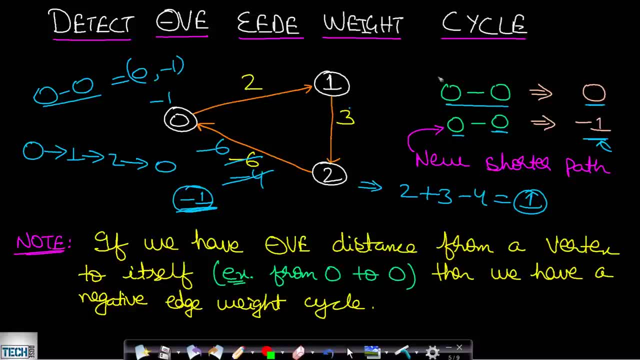 edge weight cycle because we need to check that the self distances from the same vertex to the same vertex should always be same. so you can see that it is a negative edge weight cycle and if we 0 and not less than 0, if you find any vertex to vertex distance, that is, from any vertex to the 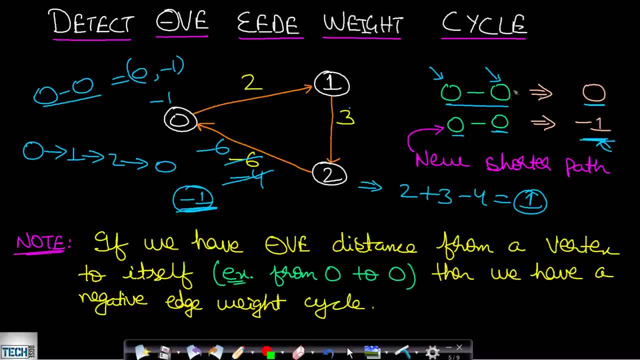 same vertex distance as negative, then that indicates that this graph will be having a negative edge weight cycle, and so shortest path cannot be found. so the thing to note here is if we have negative distance from a vertex to itself- example, from 0 to 0 in this case- then we have a 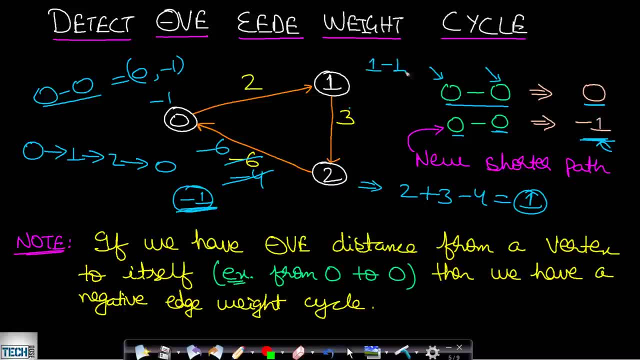 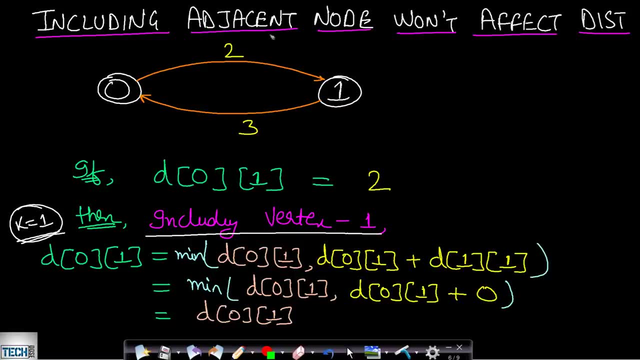 negative edge weight cycle for this graph here, one to one distance, as well as two to two distance will also come out to be negative. now, uh, the important thing to note here is including adjacent node won't affect the distance values, so let us assume that you already know the adjacent. 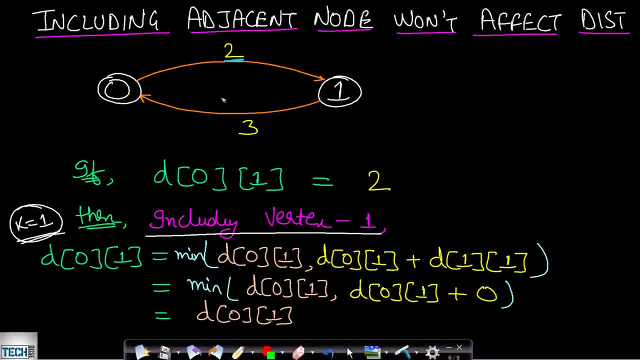 distances from 0 to 1. okay, and that is equal to 2.. so we have written the distance from 0 to 1 as 2.. now in the floyd-warshall algorithm, you will have to include each and every vertex one by one. 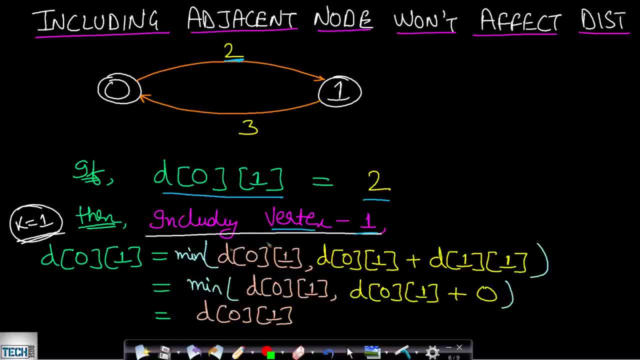 so let us assume that we are including vertex one, and now you will have to include each and every vertex one by one. so let us assume that we are including vertex one and now you want to find the minimum distance from 0 to 1, and already known distance from 0 to 1 is 2.. 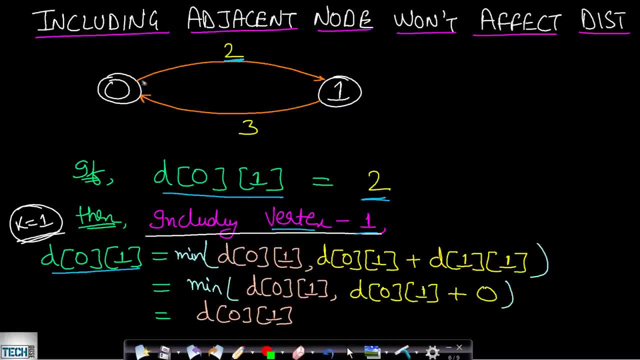 now, initially, before starting the algorithm, we know the distances for all the adjacent vertices. okay, therefore, we already know that the distance is 2.. now, since we are including an adjacent vertex which is 1, therefore, the distance values will not get updated. and how is that happening? let us see here this formulation. i had already shown you that from 0. 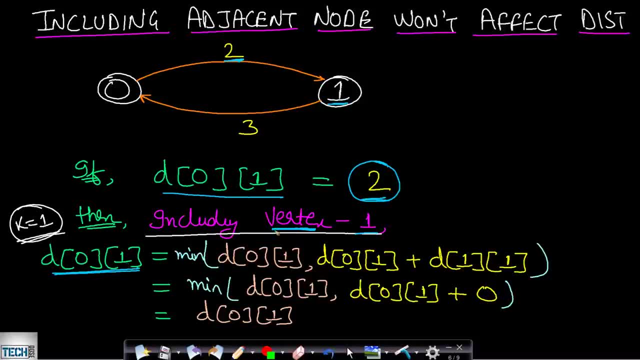 from 0 to 1. if you want to find distance, and if you are including this vertex 1, then that will be nothing but minimum of already known distance, that is, d of 0 to 1 comma, the distance from 0 to 1 plus 1 to 1.. so in this case you already know that. 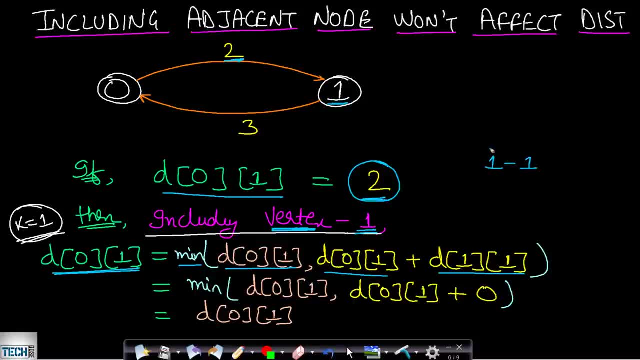 when you are not having any negative edge wet cycle. so the distance from the same node to the same node will always come out to be zero. so d of one to one will be zero. so this is as good as saying minimum of distance from 0 to 1 comma distance of 0 to 1. so this is basically the same. so the 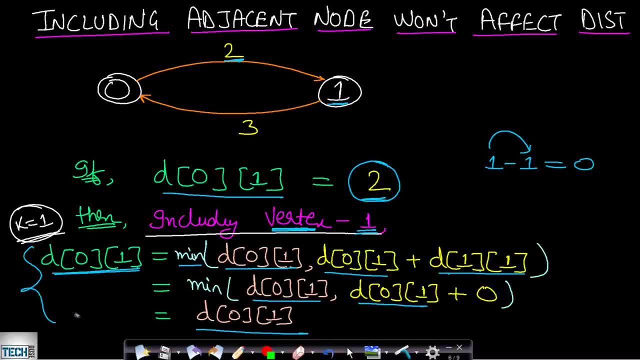 distance values will not get updated. this is the proof for that. okay, therefore, you can see that including adjacent node won't affect the distance values for the adjacent vertices. so this is one important point while solving this algorithm. so let us take an example in order to understand. 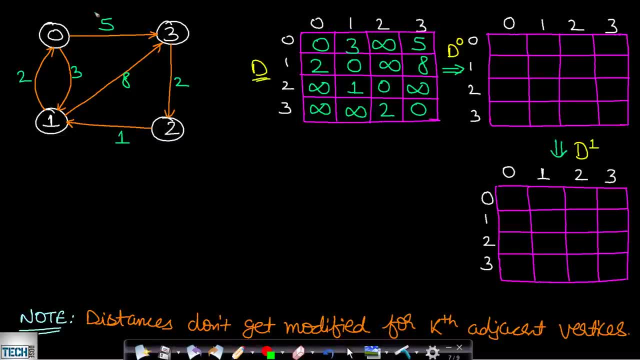 this algorithm. so i have taken this example having four vertices, so this is having six number of edges. now what i will do is, first i will make the matrix, which will be having the information about each and every distance values, and these distance values will be for adjacent nodes only and if the 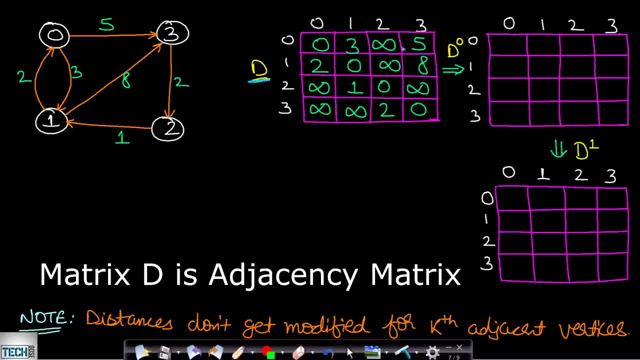 nodes are not adjacent, then actually we will be filling it with infinite value. now, in this case, for zero to three the value will be five. okay, so for zero to three the value is five here, but from three to zero it will be infinity, because then is no direct edge from 3 to 0. so by adjacent i do not generally mean that it is side by side. 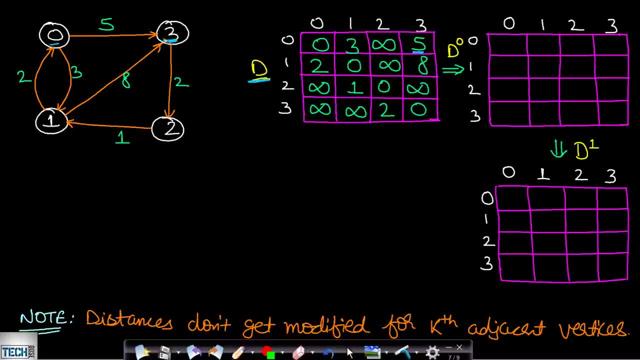 but i mean that there is a direct edge from the given node to the destination node. okay, so in this case, from 3 to 0, there is no direct path. therefore, for 3- 0 we will have value as infinity. okay, i hope you understood it now. there are no self loops, so all the diagonal values will be 0. 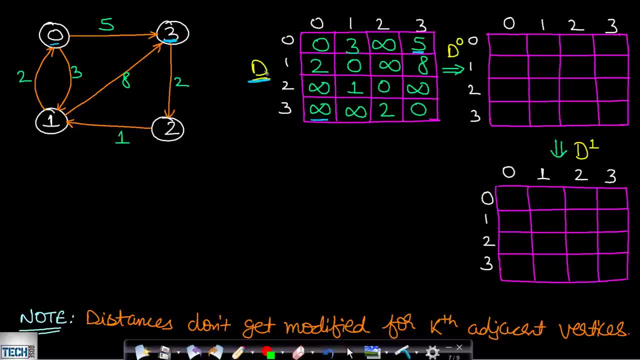 so this is also one point to remember now, once we have formed the distance value matrix. so this is just by taking the neighboring vertices, we will try to include each and every vertex one by one. so, since there are four vertices, we will be including each vertex one by one. so we will be 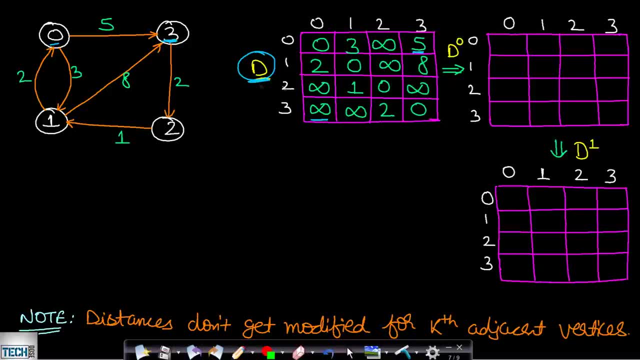 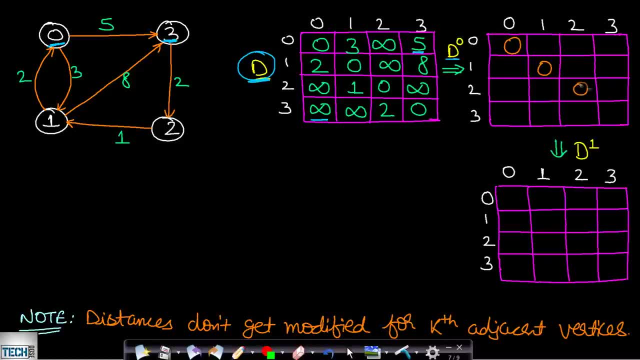 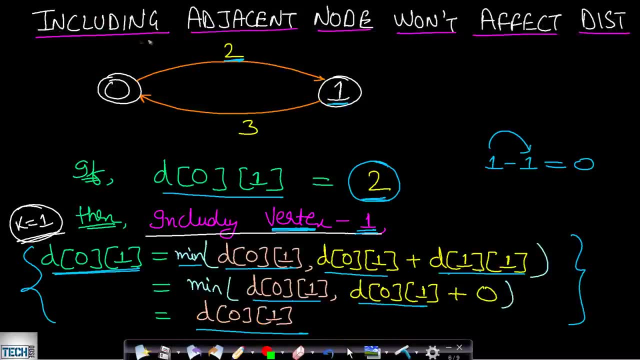 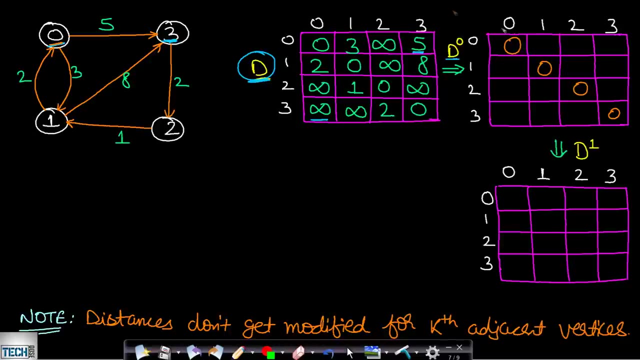 self loops. so all the diagonal values will be zero. okay, and now, since we are including this vertex, zero. so according to the previous algorithm which i had explained, including adjacent node won't affect the distance. so whatever is adjacent to zero, those all values will remain the same from. 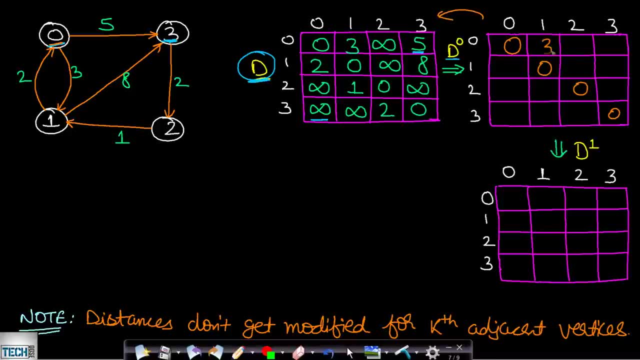 the previous state. okay, so we will simply copy this three, infinity five and this two infinity and this infinity. okay, now, whatever values are left should be filled. now. the distance values from 1 to 2 will be equals to distance of 1 to 2. it will be equals to: 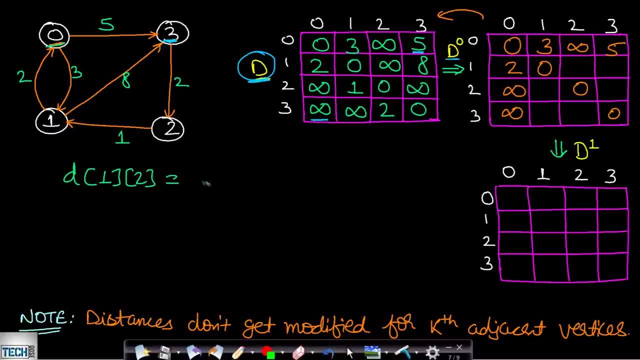 since we are including this node 0. therefore, this will be equals to minimum of distance of 1 to 2, which is already known distance comma, and that will be taken as distance of 1 to 0 plus distance of 0 to 2. okay, so this is the formulation. 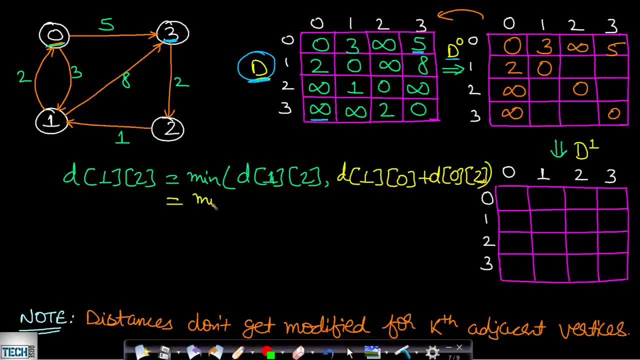 now, what will be the value in this case? it will be minimum of distance of 1 to 2. 1 to 2 distance is infinity, so this will be infinity comma. 1 to 0 distance is 2, so this will be 2 plus 0 to 2 distance. 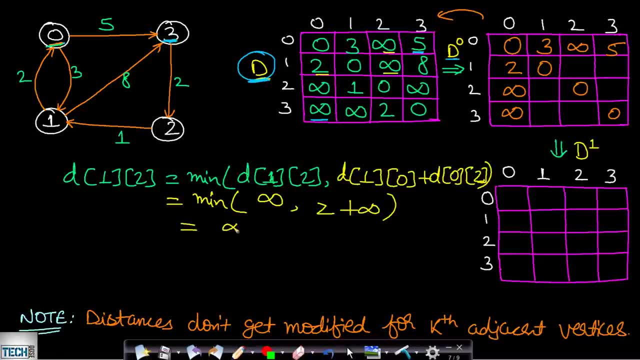 is infinity, so this is infinity, so it will come out to be infinity. okay, therefore, we will fill here infinity. like this, we will be filling for each and every value. now let us fill for the next value, which is for 1 to 3, which is for 1 to 3. 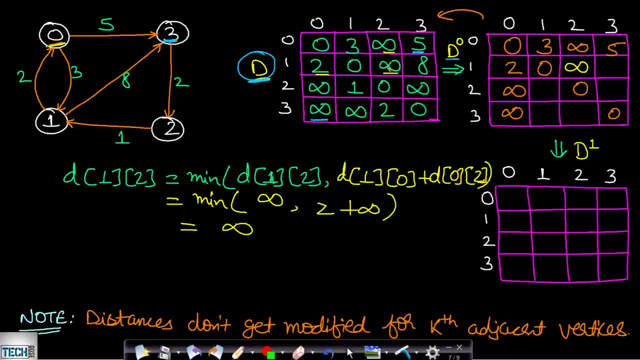 including this vertex, 0. so for 1 to 3 the already known distance is 8, so we will be taking minimum of 8 comma and then we will be taking from 1 to 0 and 0 to 3 according to this formula. so from 1 to 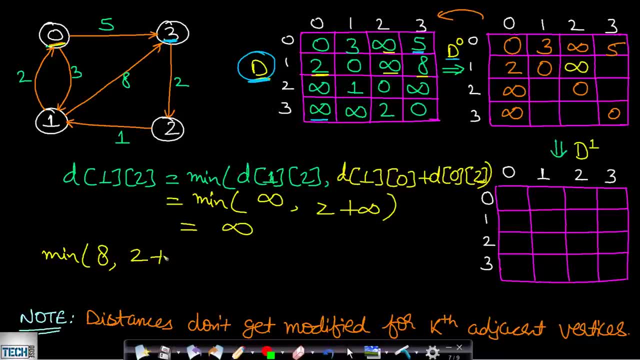 0- 1 to 0, the value is 2, so this will be 2 plus. and from 0 to 3- 0 to 3, the value is 5, so this will be 5. now it will come out to be 7, so this will be replaced with value 7. you can see that previous. 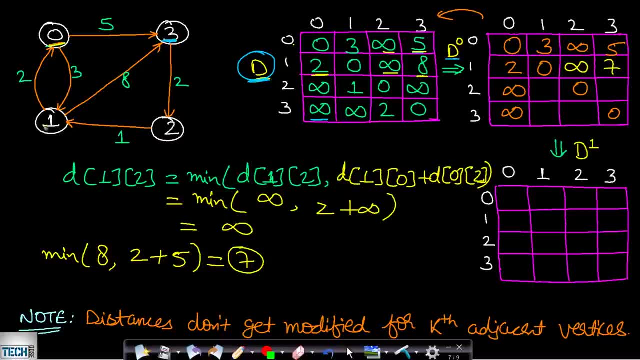 3 gonna be replaced with 0, so that 1 the same as 7. right now. we are taking the same note and now, if we fill the triggers code, we will receive 2 and we will get the same result that the number of out of the order graph is 8. so that is, changes run like this, which: 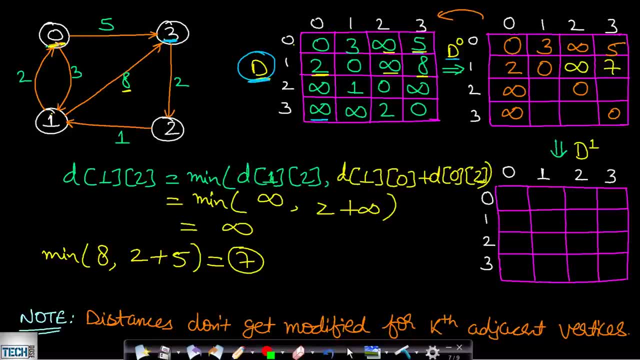 will help us to define the number of running three through five and we will get infinite part and also now the other done especially. just to show you, the concept of y can be transferred inside in one Say: the three is a wonderful воaving and it will also be. 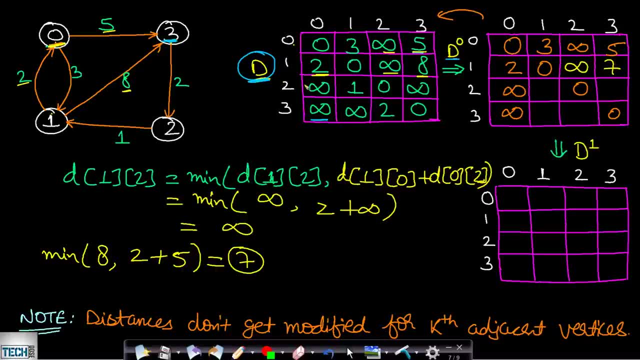 possible that we will be able to see, as if we go and if we want to be able to see the sun. now let's see this node: 0 is considered reducing the space between 2 and 0. we already said, as 0, 0 is considered increasing the greater its weight isn't the 10th clock. this 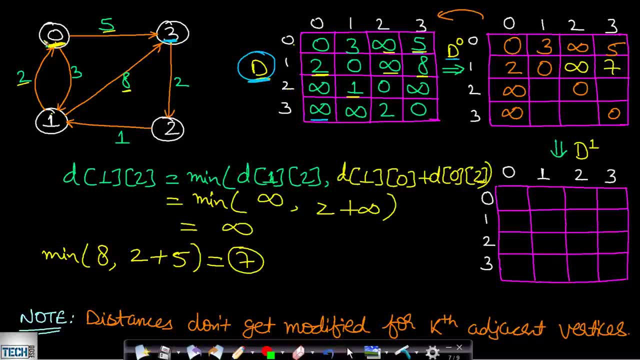 step will still still not be fulfilled until you are able to see the final value. we shouldn't. then the distance will be from two to zero and from zero to one. so from two to zero, the value is infinity. so since this edge from two to zero is infinity, we can say that this is infinity, and so 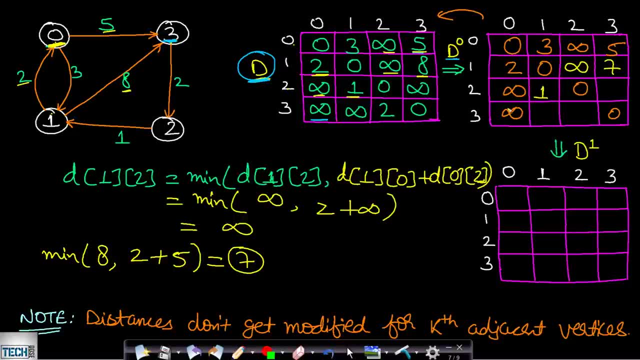 this will not be included. so whatever is the value is coming, we will just paste it here, because nothing is greater than infinity. okay, now the next part is from two to three. so two to three, already known distance is infinity, so we will take minimum of infinity comma and from two to three via this: 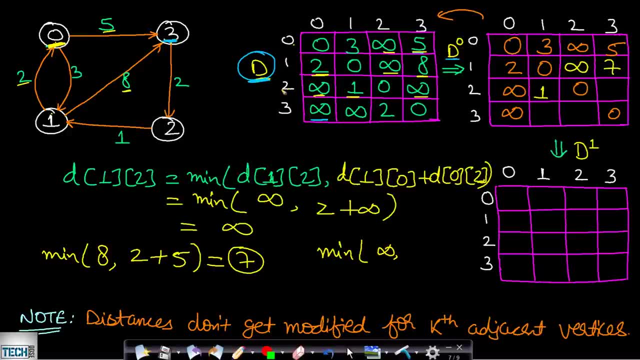 zero. it will be two to zero, and then from zero to three. so two to zero is also infinity, plus whatever the value is. we don't care actually, so this will come out to be infinity. we will write here: infinity. okay, now for this one. from three to one, from three to one. the value is infinity. now, from three to one. 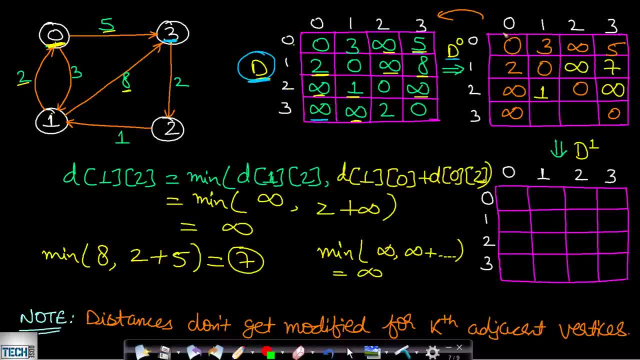 via this node, zero. it will be three to zero and zero to one. so three to zero. distance is infinity, so we don't care about the other part. actually it will be infinity, minimum of infinity, comma infinity. now we will see, from three to two, three to two, the 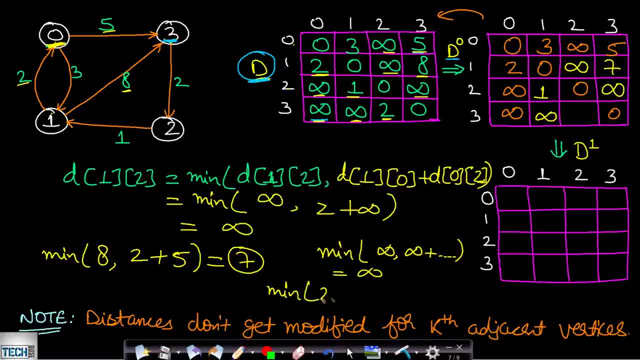 distance known is two, so it will be minimum of two comma. now, via this zero, it will be from three to zero, and then from zero to uh, this two. so three to zero distance is infinity, so we don't care about the other part. it will come out to be two. okay, so the distances are not changing. 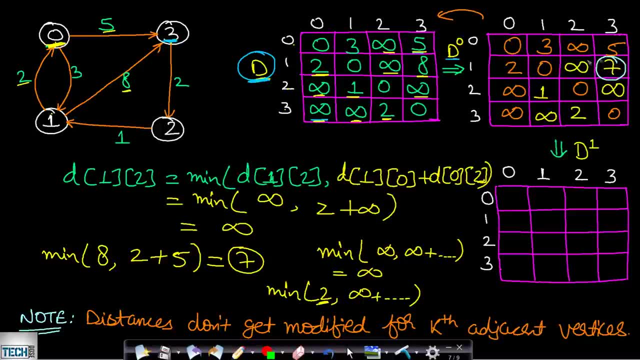 so in this case we have just a single change, that is, this part. it was eight, from one to three, and now it is changed to seven, from one to three distance. okay, so we are done with including this node zero, and now we will include the next node, which is node one. so when we are including 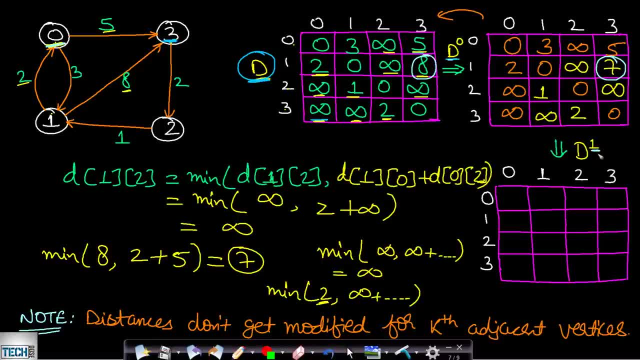 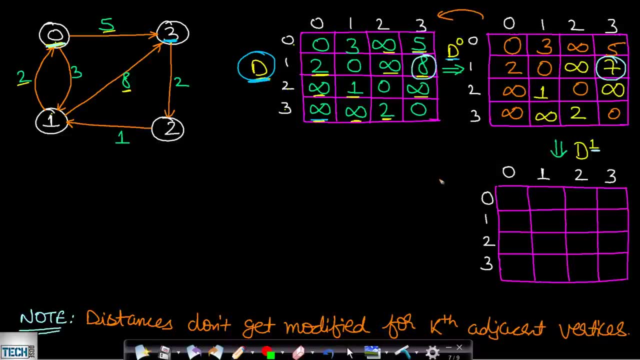 this node one, then node zero is already included. therefore, whatever is processed and answered here will be containing both node zero and node one. okay, now, in this case as well, we will first be including all these values as zero, since there are no self loops. now, since we are including node. 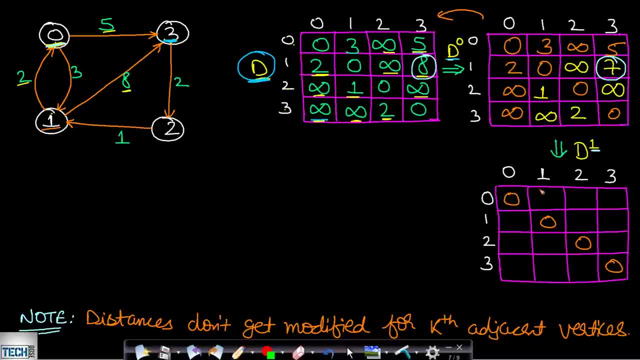 one here. therefore, all the adjacent nodes will not be changing value, so we will simply be copying the values here from the previous state. so this will be infinity, and for this one this will be two, zero, infinity and seven. so this will not be changing the values. so now we will be processing. 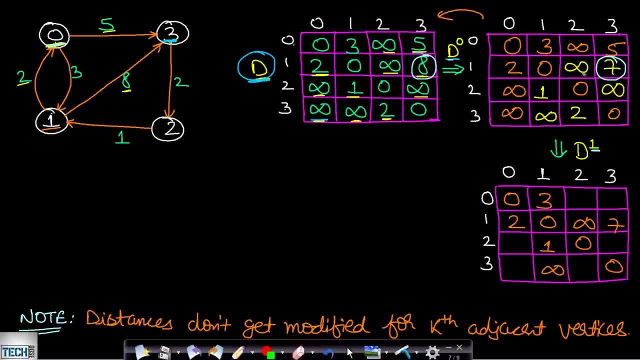 for the other parts. so for this zero to two, the value already present is infinity. in the previous, now, in this state, uh, it will be via this one. so already present distance is infinity. we will be taking minimum of infinity comma. we are finding from zero to two via one, so this will be zero to. 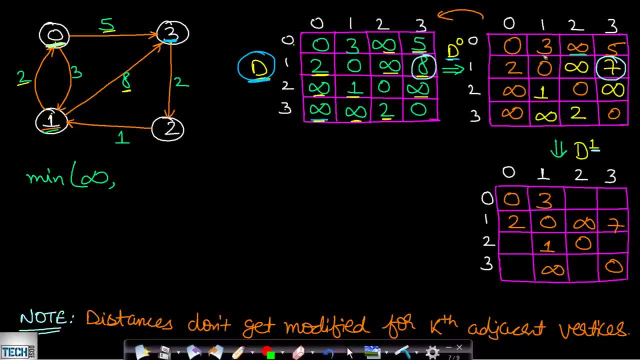 one and one to two. so from zero to one the distance is three, so this will be three plus, and from one to two, one to two, the distance is infinity, so this will come out to be infinity, so we will write here: infinity. now for zero to three, already present distance is: 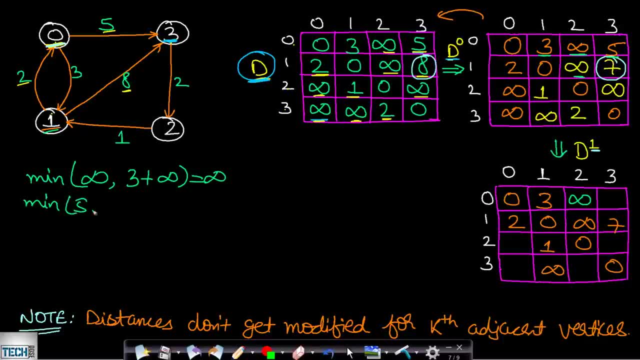 five. so this will be minimum of five comma. now we are including this one, so it will be from zero to one and from one to three. so zero to one distance is three and one to three distance. one to three distance is seven, so this will remain as five. okay, so i will write here five. now let us 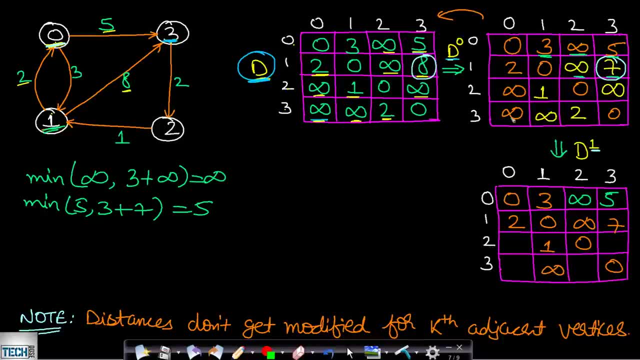 see the next part, which is from two to zero. so two to zero. already present distance is infinity. now this will be minimum of infinity comma. now we are finding from two to zero via this one. so this will be from two to one and then from one to zero. so two to one distance is one, and then from one to zero the distance is two. so this will 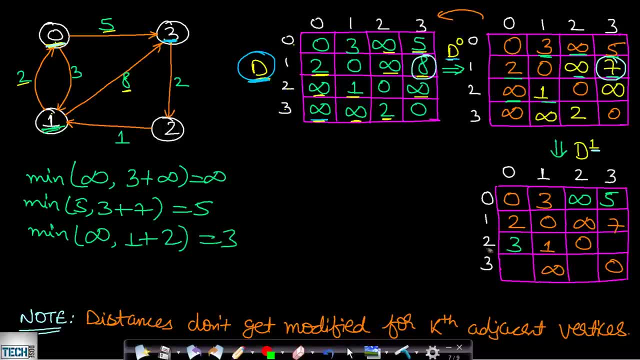 come out to be three. therefore, we will write three here now. the next part is from two to three. so from two to three. already known, distance is infinity, so this will be minimum of infinity comma. and then, uh, we are finding from two, two to three via this one. so this: 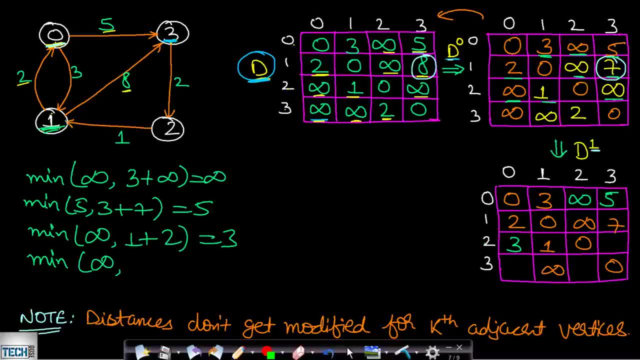 will be two to one and then one, two, three. so two to one distance is two to one, is one, and one, two, three is seven, so this will come out to be eight, so we will write here eight. okay, now you can see that this one has changed here and this value is also getting updated, okay. 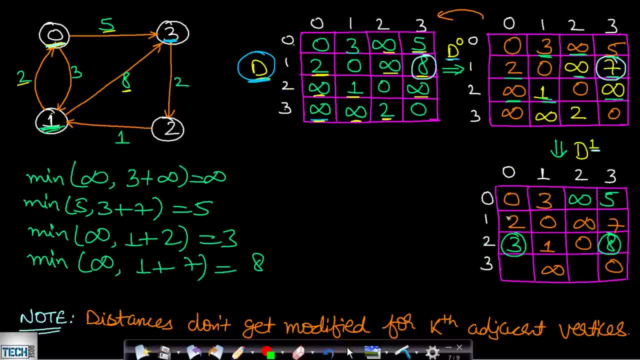 now we will also see for this three to zero. so for three to zero value is infinity. so we will take minimum of infinity comma. and now, since one is included, so we will see from three to one, and then from one to zero. so for three to one value is infinity. so we don't care about the second part. 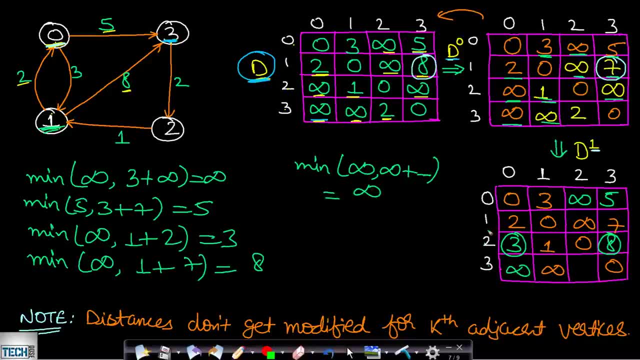 it will come out to be infinity. we will write here infinity. now we will see for three to two. so for three to two, value is two. so this will be minimum of two comma. and then we are finding from three to two via this one. so this will be from three to one, and then from one to two. so three to one value is 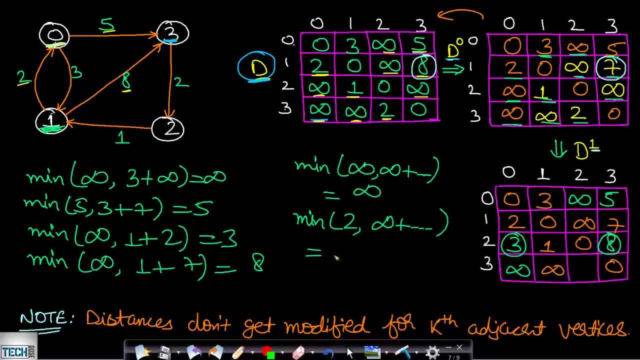 infinity. so we don't care about the second value. it will come out to be two, so this will be two here. okay, so after including both the nodes, zero and one, this is our shortest path. matrix- okay. so like this, we will keep repeating and include all the vertices and whatever matrix come at last. 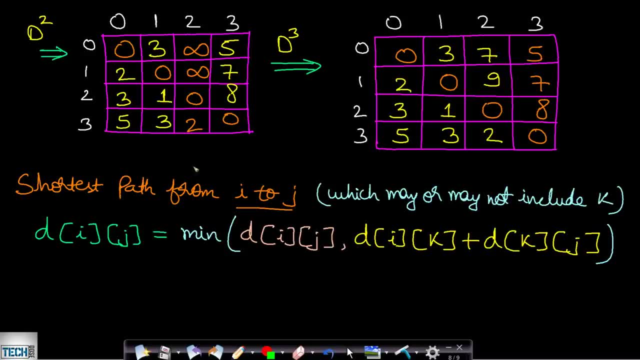 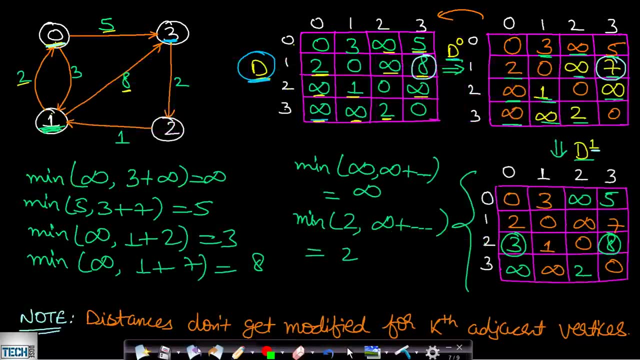 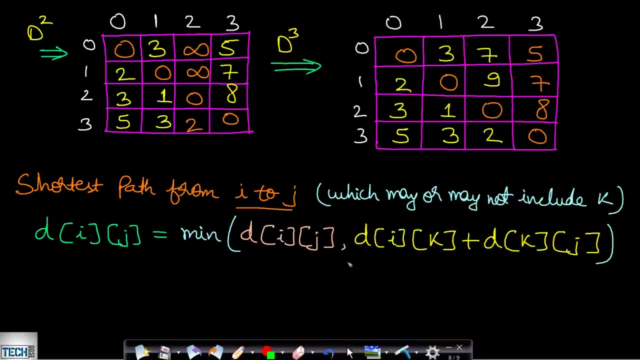 will be our final all pair shortest path. so if we solve it, then this will be the final matrix. okay, now then, so you can see that this algorithm works. so you can see that in this algorithm, the shortest path from i to j including. so in this algorithm, you can see that the shortest path from i to j. 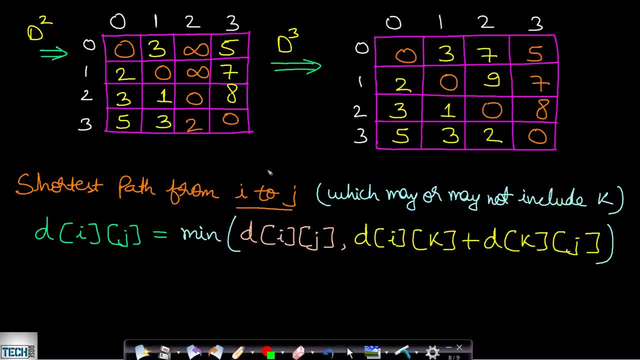 including a node k. so in this algorithm, one important point to note is: if you are finding the shortest path including a node k, then that may or may not be the shortest path or may not include the node k. so in this algorithm, one important point to note is that 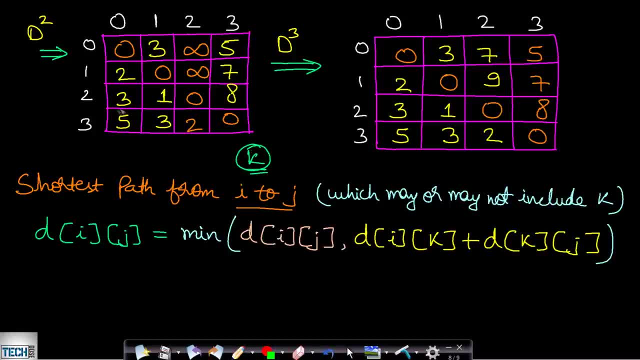 if you are including a node k. in this case we had included node 0, 1, 2 and 3. so if you are at the kth node and you are willing to find the shortest path, if you have the option of including this node k, then the shortest path value may or may not include the node k. so whatever formula, 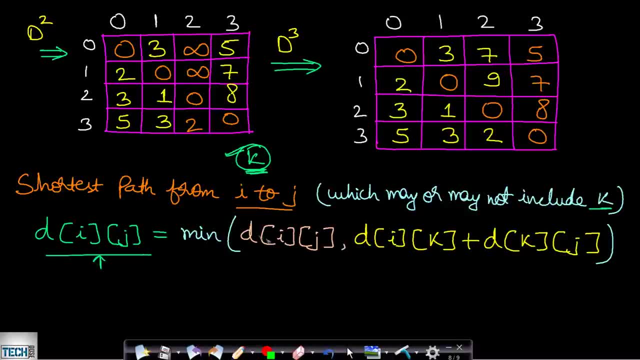 is written here, that is, the minimum distance from i to j will be equals to not including the current node, which is k. otherwise, including the current node will give us the answer. so this first part is actually saying that we will be skipping this node, we will not be including this node k, and the second part is saying that we will be including this node. 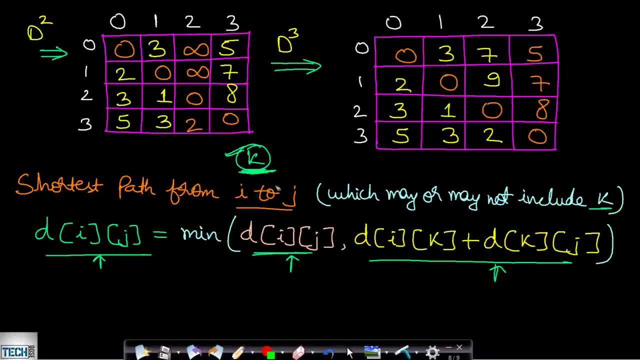 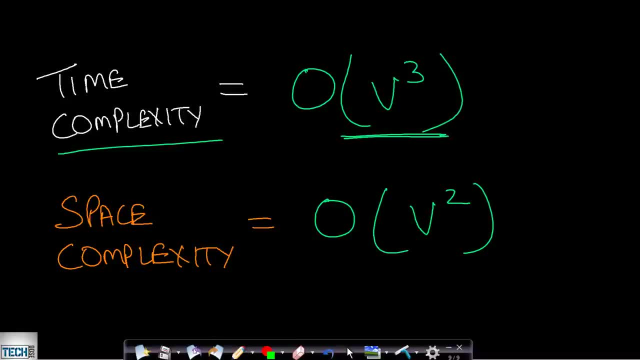 k okay. so this is one important thing to remember now, having seen this algorithm: what will be the time complexity? well, the time complexity will be order of v cube. and why is that? because we are actually including all of these vertices, and we are actually including all of these vertices, and 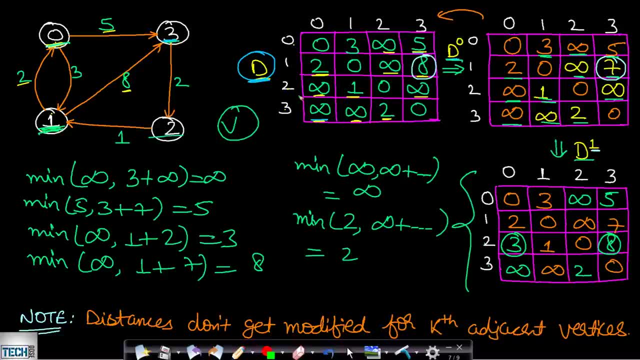 he says each and every time: okay, so there are v number of steps for inclusion and now you are filling the matrix, which is of size v, by v, so this matrix size is v square and we are filling it v times, so it will be v into v square, which will be v cube. okay, so the space complexity will be. 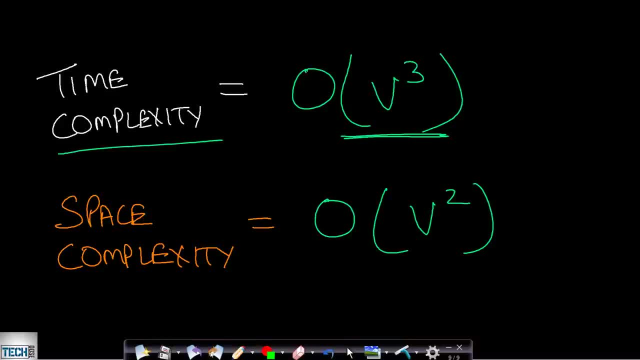 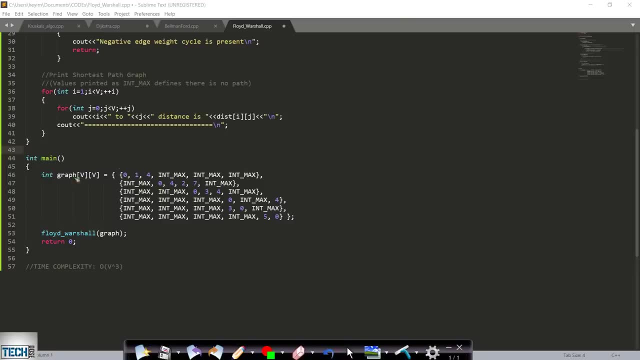 v square, since we are taking a matrix of v square size. so this is the time and space complexity analysis. let us now look at the code. now, this is the simple floyd-warshall code. in this case, i have made a graph and whatever you are seeing as 0 is basically nothing but. 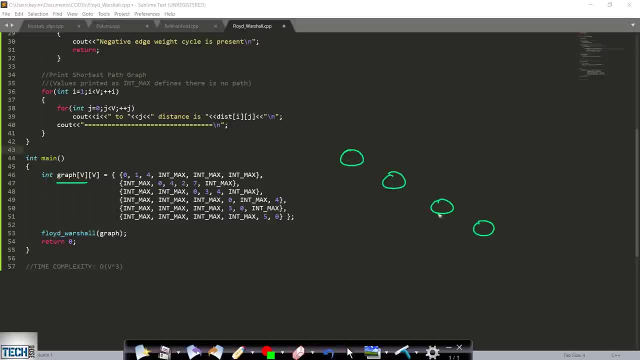 the diagonal values. that is, there is no self loop, so it will be 0 and whatever you are seeing as integer maximum, it indicates that we do not know the distance from a given vertex to a certain vertex. so this integer maximum is saying that we do not know the distance from 0 to this is 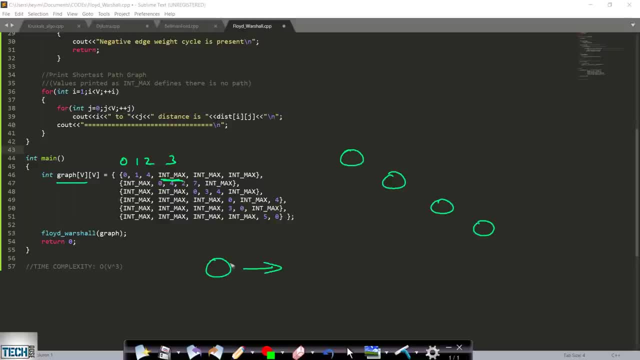 a vertex: 0, 1, 2 and this is 3, so we do not know the distance from 0 to 3. okay, so that is why we are writing integer maximum. so, according to this algorithm, initially we will only be knowing the distance values to the adjacent nodes, okay, and then we will keep. 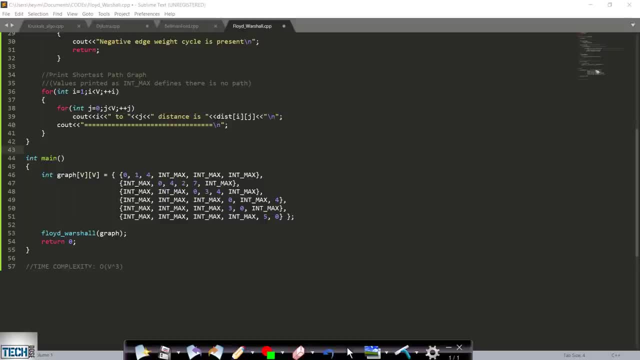 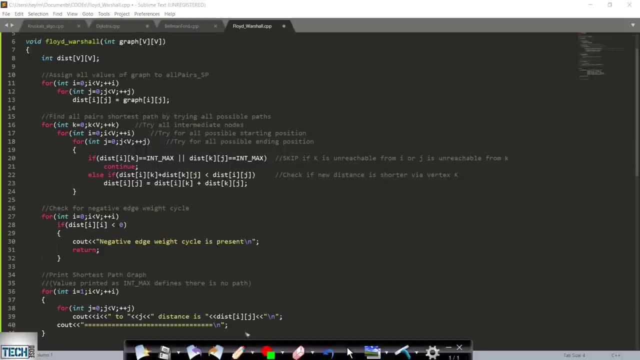 including each and every vertex one by one in order to find the shortest path. so let us now look at the algorithm. so this is the floyd-warshall algorithm. in this case, i have fixed the number of vertices to 6, so when we are taking this, 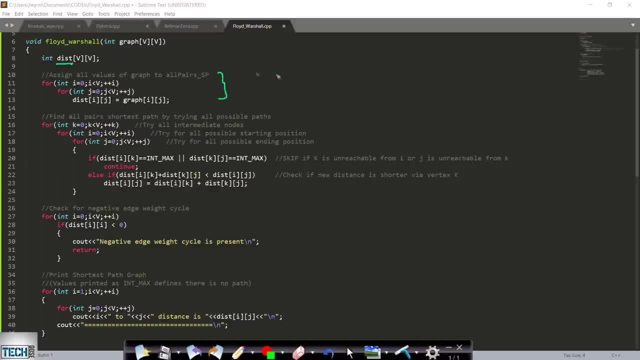 distance values, then actually we will be copying all the adjacent node values. so at node values are already stored in this graph, so we will be taking it down and copying it in distance matrix. now the distance matrix will be finally giving us the shortest path between all the 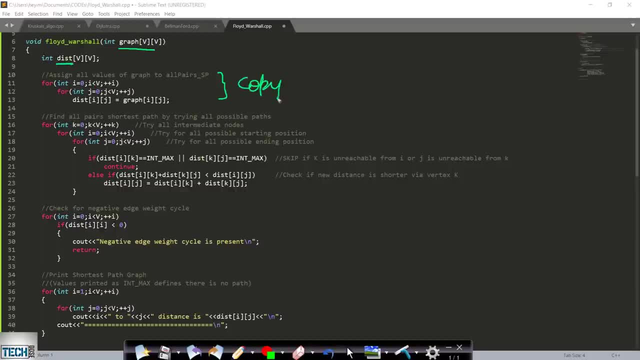 pairs of the graph. so first we will copy. so this is the copying step. now we will find all pair shortest path by including each and every vertex one by one. so this outside for loop is basically our k value, which is including each and every vertex. and since we are including a vertex, 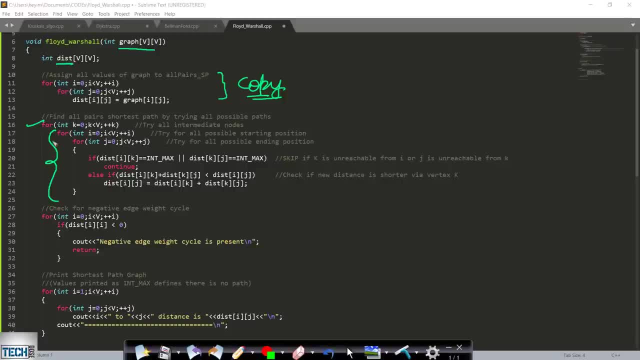 therefore, we will be calculating the shortest path when we have the option of a given vertex being included. so we started with vertex zero, then we included this vertex one, then two and then three, and then we stopped. okay, so we will be including each and every vertex one by one. 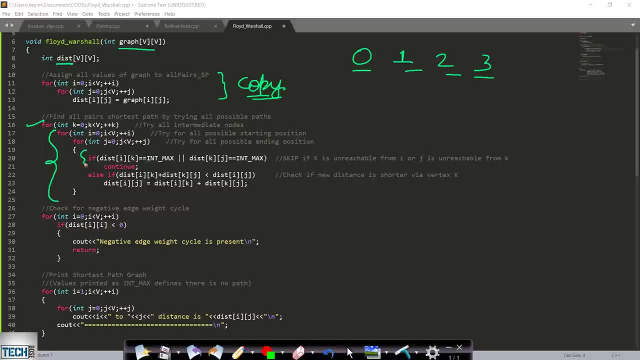 and in this case, this is the option like: if we are including a vertex, then let us say we were knowing the distance value from zero to two. now we have an option to include this one, so we are including this one, and then we are including this one, and then we are including. 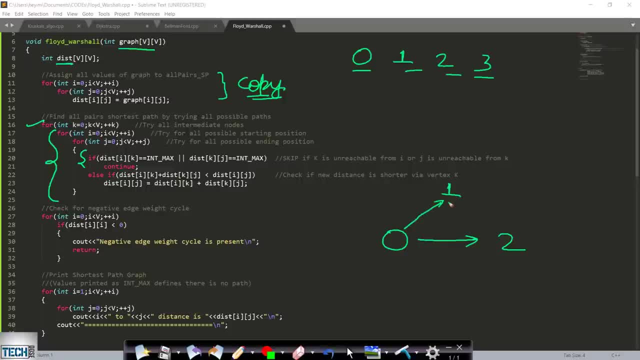 this one. so if the distance from zero to one is known and from one to two is known, then only we can compare the distance values. okay, but if the distance from zero to one is infinity, that is, we do not know, or the distance from one to two is infinity, then we can say that since we do not know, 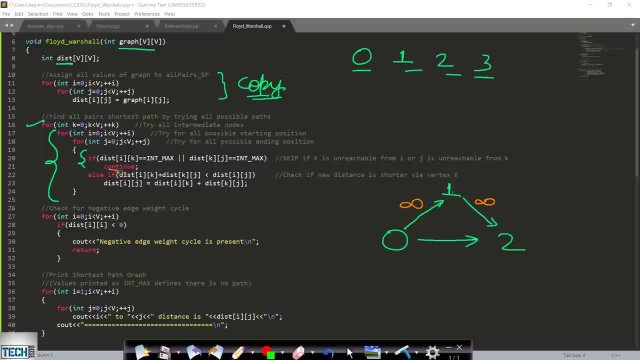 the distance values. we cannot compare it and therefore we will continue, that is, we will skip this step. so i will repeat: if we have no knowledge of the distance value from 0 to 1, or from 1 to to 2 or both of them, then we will simply skip the step. otherwise, if the values are known, let's say: